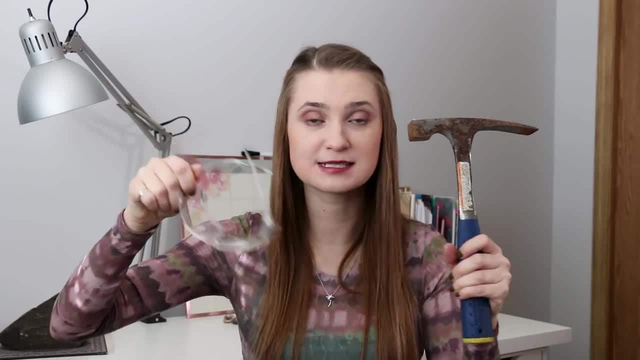 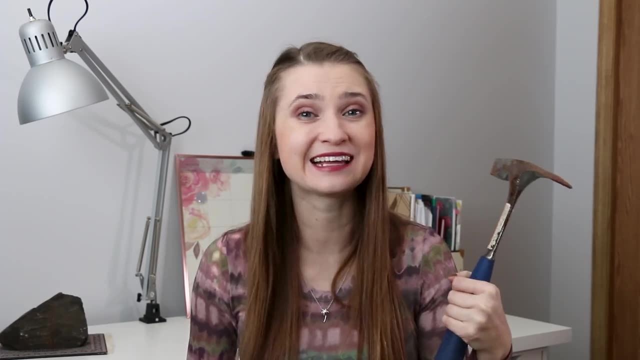 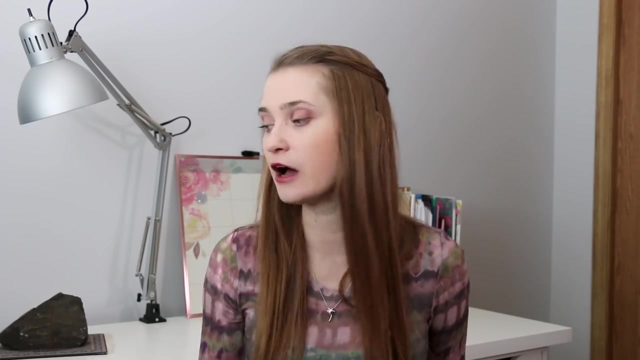 And of course with the hammer comes goggles or glasses. I have seen geology students hammer at rocks without eye protection and one student had one. I have seen geology students hammer at rocks without eye protection and one student had one. One student had a rock chip land in his eye and he had to go to the hospital. so don't be that person. safety always comes first, because it's all fun and games until it happens to you and then it's not fun anymore. 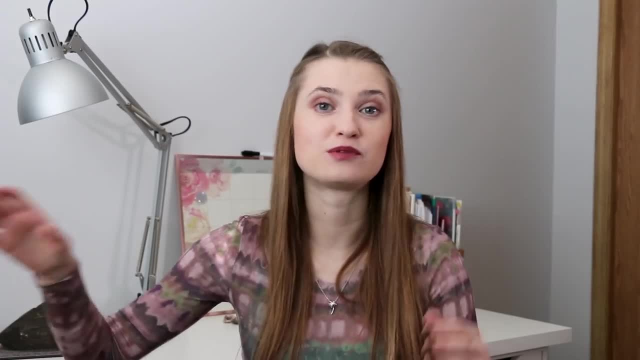 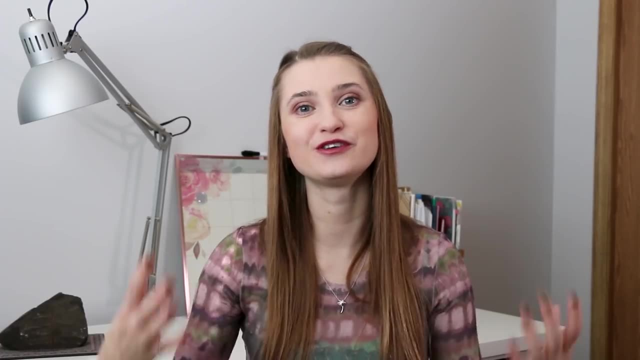 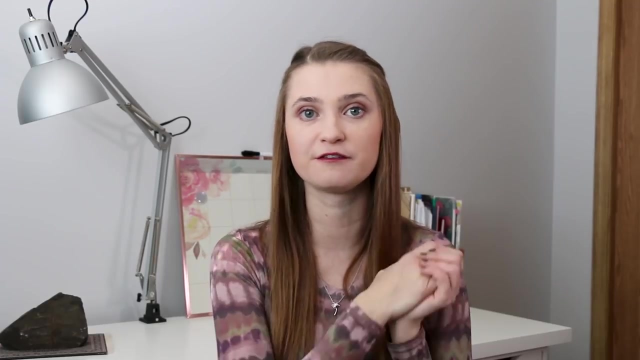 So, but hammer is number one on my list. The next thing is Brenton compass. Now, I don't happen to have one with me because I was lucky enough our school would lend us Brenton compasses during field school. So when we go away they will give us, assign us, a compass for each student, and then we'll just give them back to school at the end of the field course. 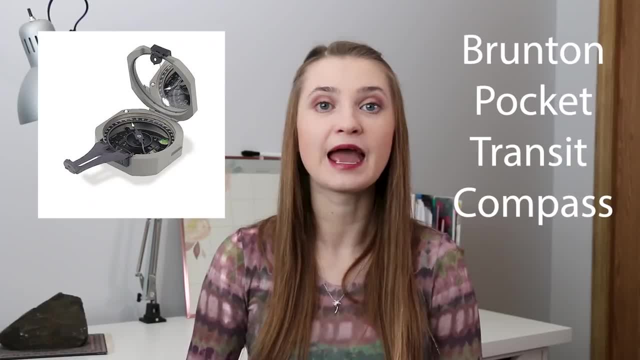 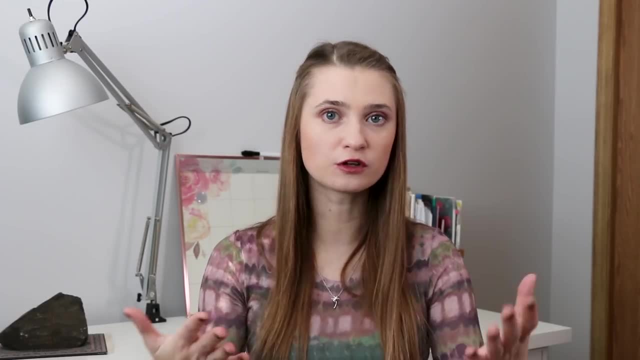 Now, if you don't know what a Brunton compass is, it looks like this, And Brunton compass is specifically used primarily by geologists, And the reason it's useful is because it allows you- not only it allows you- to determine direction. 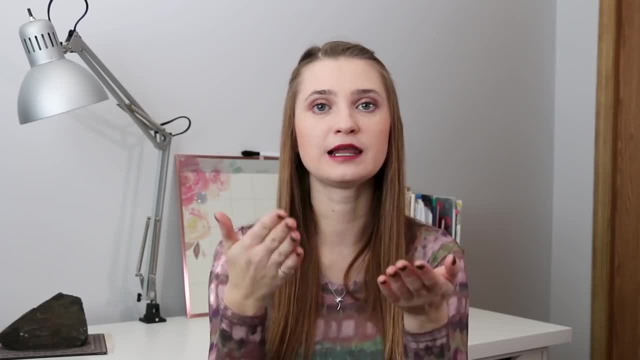 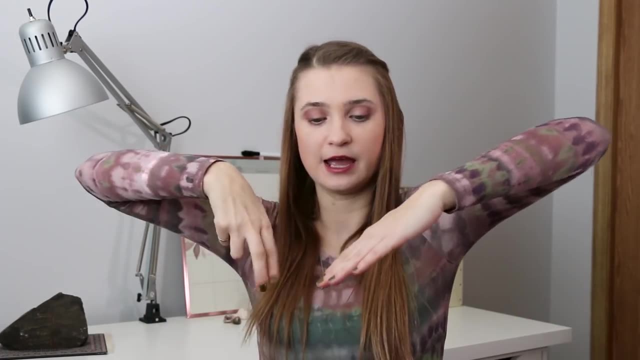 like north, south, east, west, right. But it also allows you to measure strike and dip. And if you don't know what a strike and dip is, if you imagine a rock surface like this, so say, this is a rock, and you're walking along and you want to measure this angle relative to the horizon. 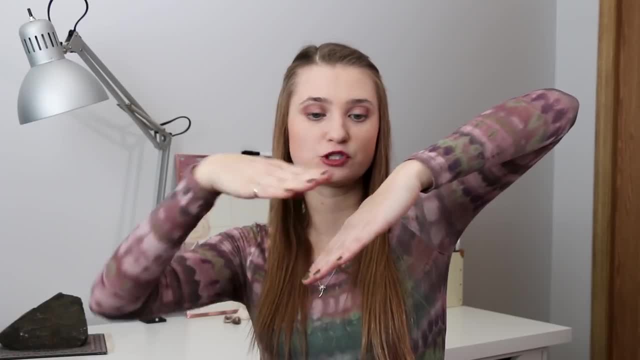 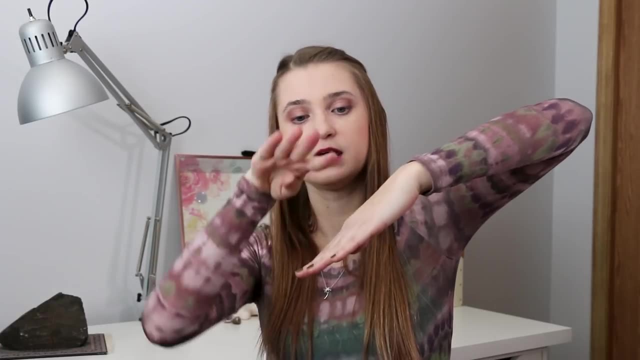 then that Brunton compass allows you to do that. That's called a dip. So you would put a compass on the rock surface like this, and in the compass it will read that angle between the horizon and the angle of the rock, And it also lets you to measure strike, which is this direction. 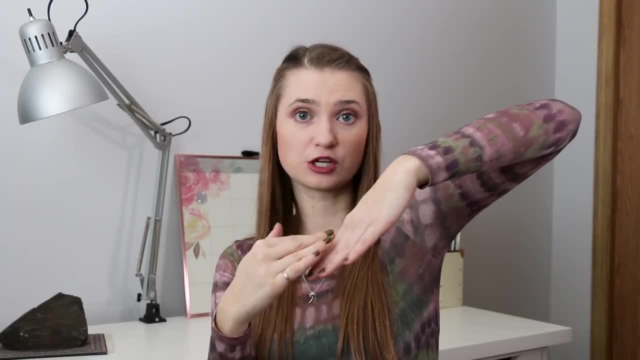 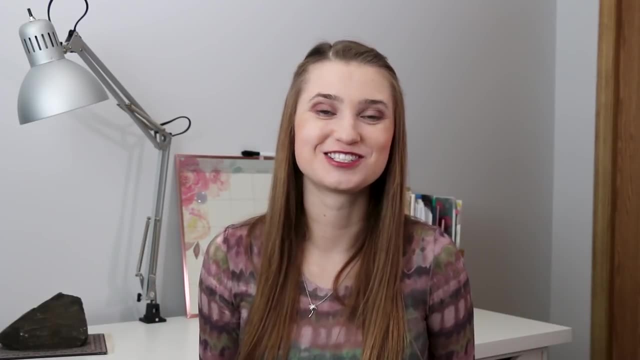 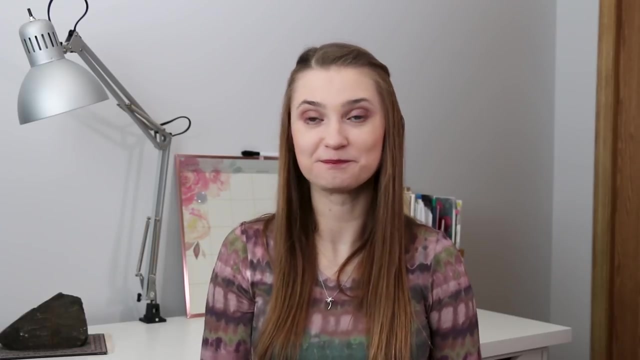 And it's basically direction of the line formed between the rock surface and the horizon line And it also allows you to measure that And it's a very useful information for geology, geology students, because you are asked to, You have to do a lot of maps of rock outcrops and such, and you must know that information. 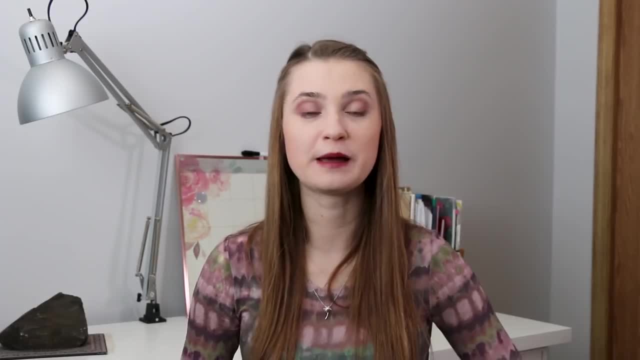 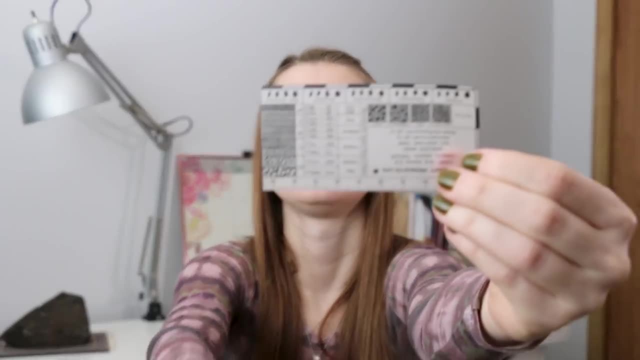 Next thing on my list, which is by far the most used by me and still used to this day, is the grain size card. If you don't know what a grain size card is, I'll see if I can, if this will focus. there you go. 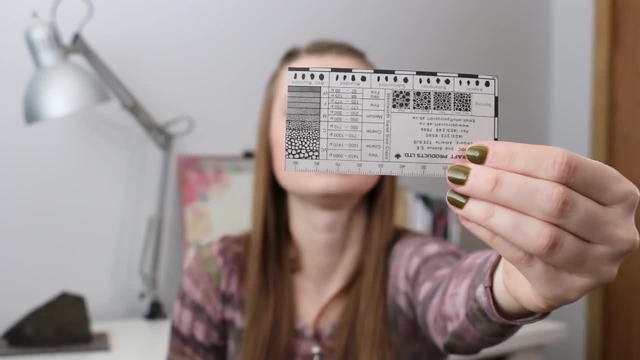 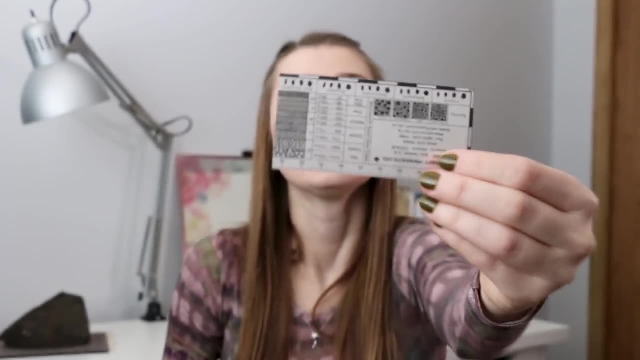 So a grain size card is used to measure grain sizes of the sedimentary rocks, also determine their roundness and how well sorted they are. Now, not only this is useful, it's useful for determining the grain size, but it's also useful as a scale. 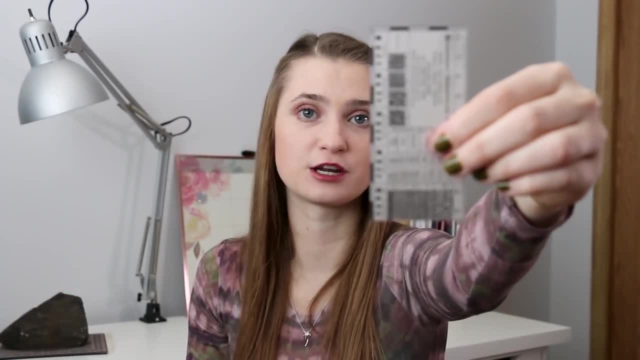 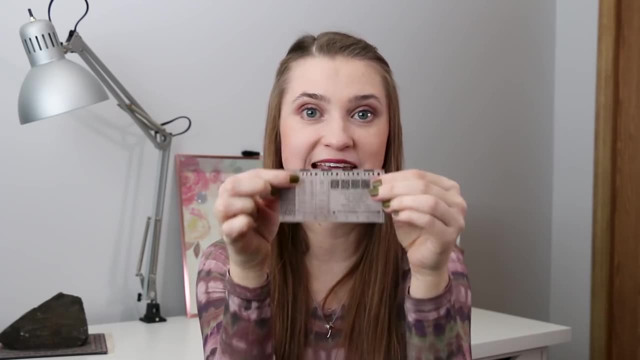 If you are doing any sort of field work, if you, even if you're not a geology student, this is gold because it comes with a scale and you know, when you're writing a report, how important it is to have a scale on your map. and this is two in one and it's perfect. 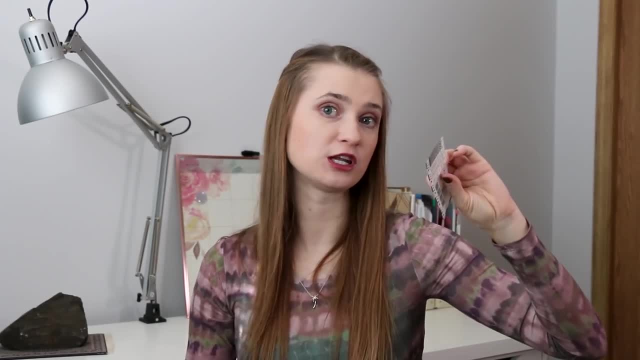 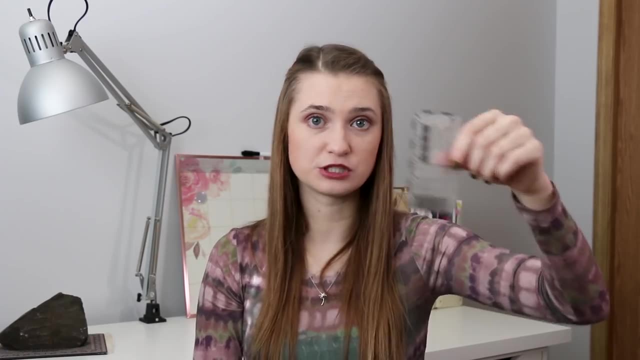 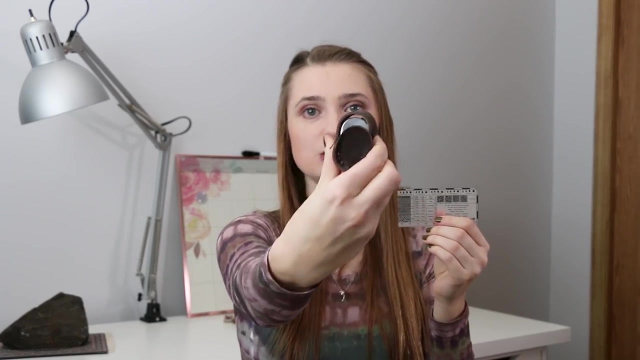 and it's small and it always comes with me And, being a petroleum geologist, I primarily worked with sedimentary rocks after during my career and I always always use this Now with the grain card. it's also important to have a hand lens, and mine comes in this. really super cute pouch. 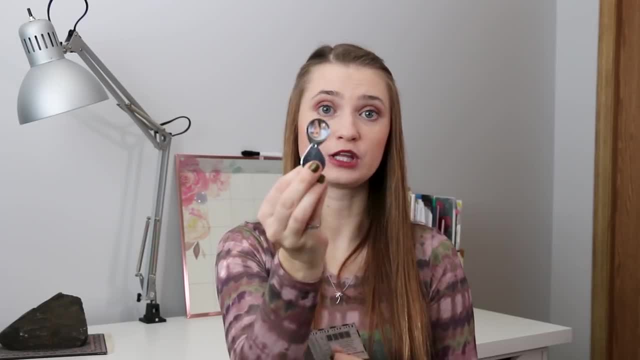 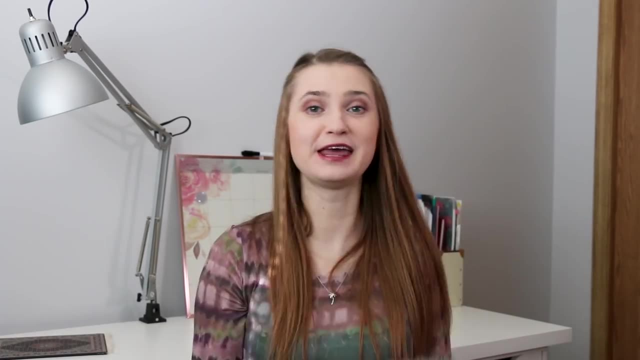 and basically that's what that is- is a hand lens that you look at the rock really close to determine the grain size. Now I'll show you, I'll demonstrate how you use it. so in the field, if you're playing the rock, 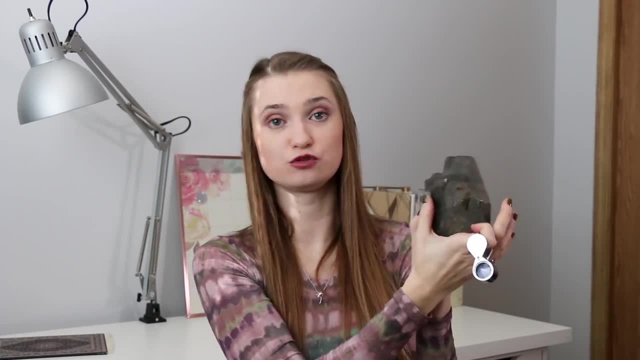 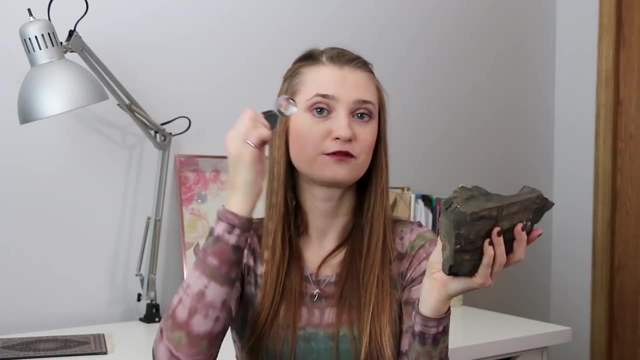 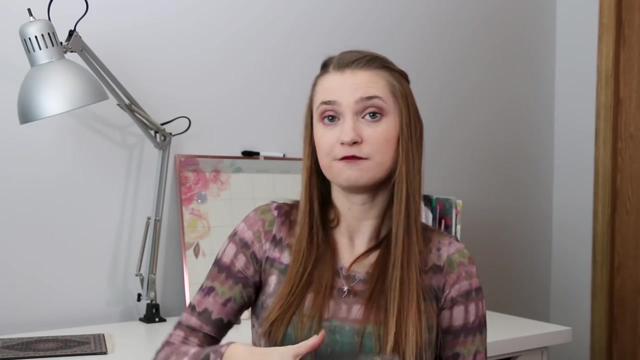 and you say, hmm, I wonder what grain size that is, because you're doing a description of it. you would put your grain size by that rock really close. you would put the lens right against your eye, go really, really close and then sort of determine the grain size of that rock. 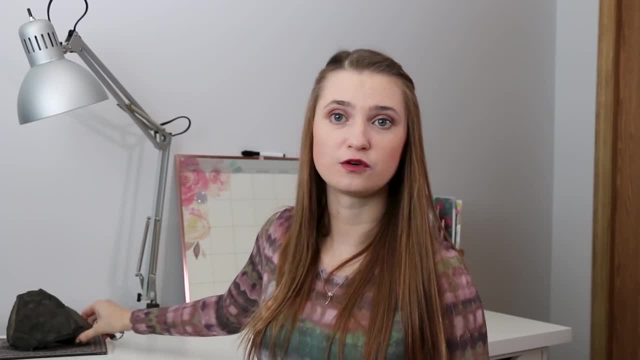 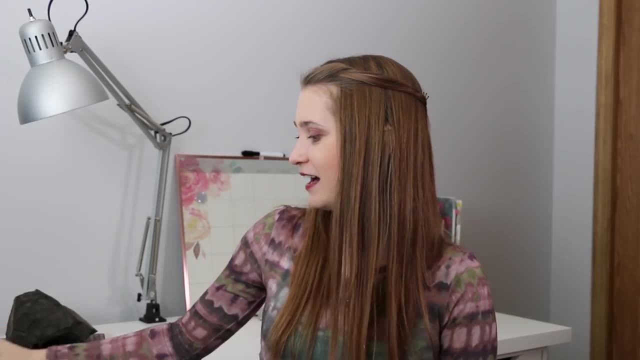 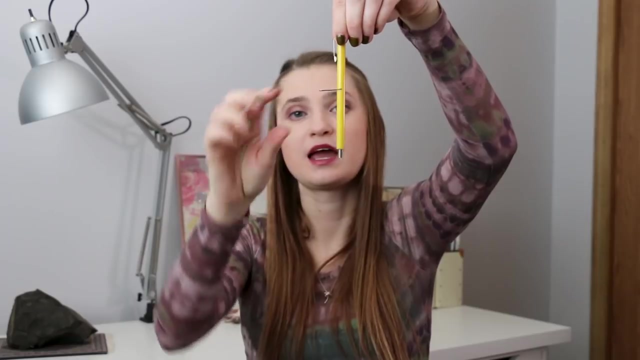 Very, very handy as well. Now, they are pretty small, so I have lost a couple of them in my life, but nevertheless. Next thing is the magnetic pen. Now, it's exactly what it sounds like: It's a pen with a magnet at the bottom and a little handle here, and what it's used for is used for determining. 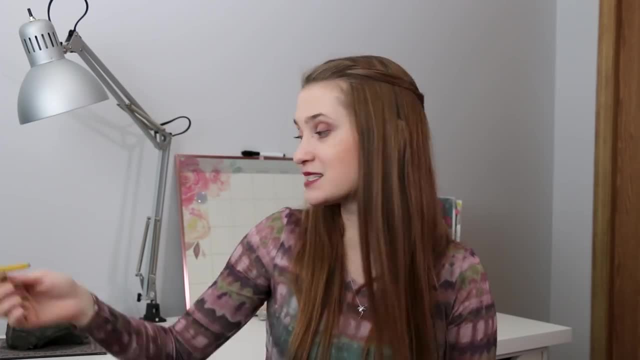 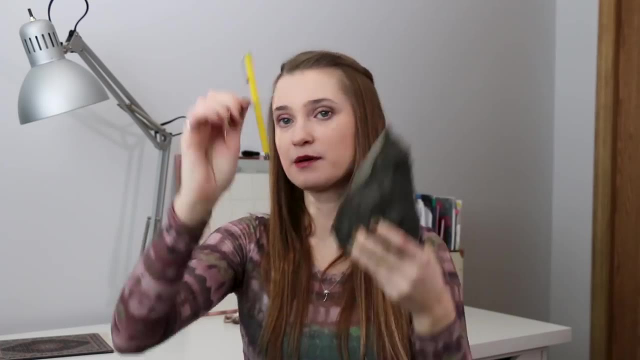 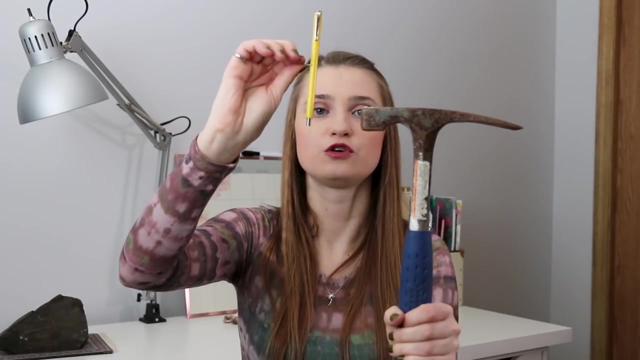 if the rock has magnetic properties, magnetic elements. Now, if the rock doesn't have magnetic elements like this one, the pen doesn't move, obviously, so nothing happens. but if you have something magnetic, like a rock- with I don't have any magnetic rock, but a hammer will do so- you can see that the pen gets attracted to it. 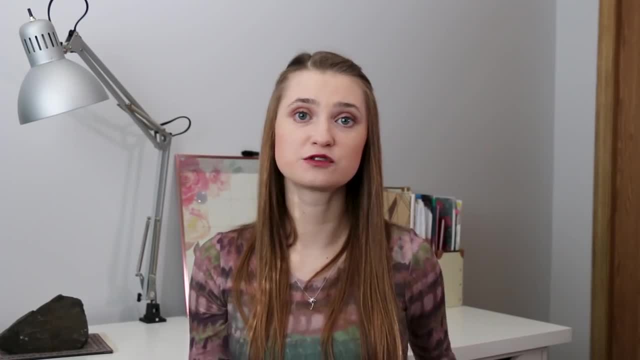 very easily and that's very useful in the field. and it's useful to have this pen instead of just the magnet. it's useful to have this pen instead of just the magnet, because when you're playing with a rock, you can't really see anything. 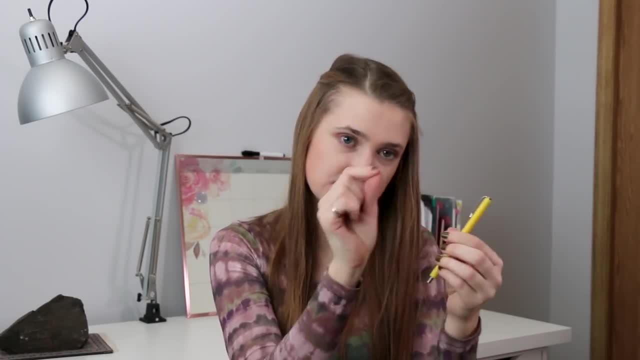 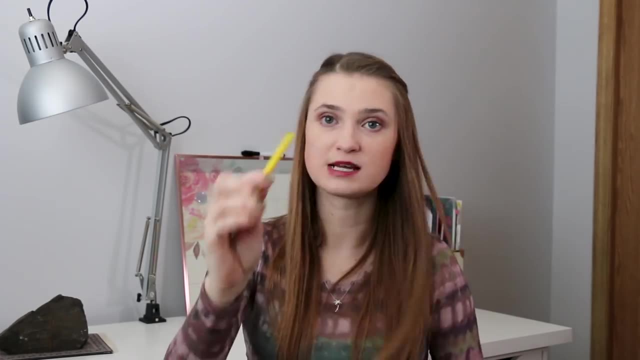 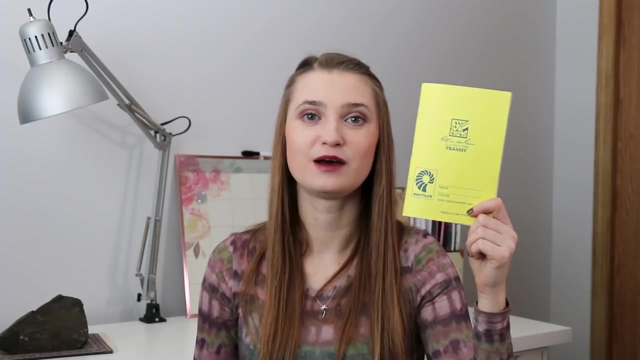 you're dealing with a big rock and you're trying, with a small magnet, to see if it's attracted to the rock. it's really hard, especially if the rock is like really weakly magnetic. um, this pen is a must. it was must for our field work as well. next thing is: uh, also very handy. uh, it's a all weather. 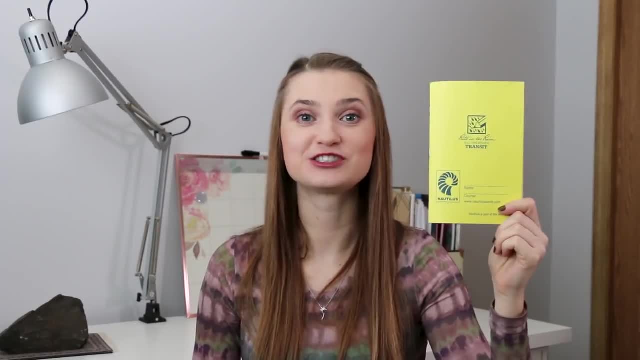 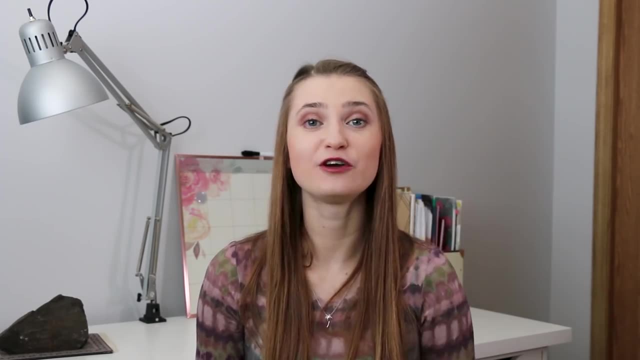 resistant geology notebook. now, if you are interested in getting one, i am giving one away. this is where the giveaway comes in. i'm giving one of those away, brand new- and if you are interested in getting this one, uh, subscribe to my channel and follow me on instagram at shylamagirl. 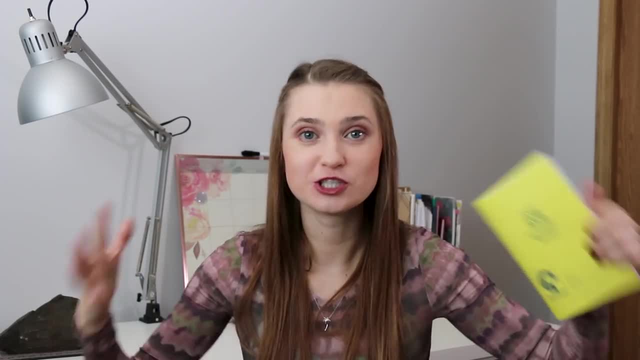 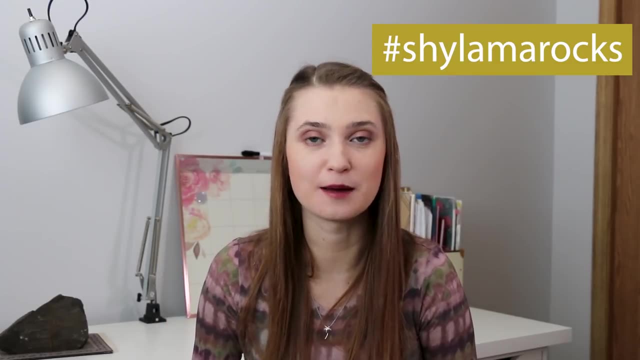 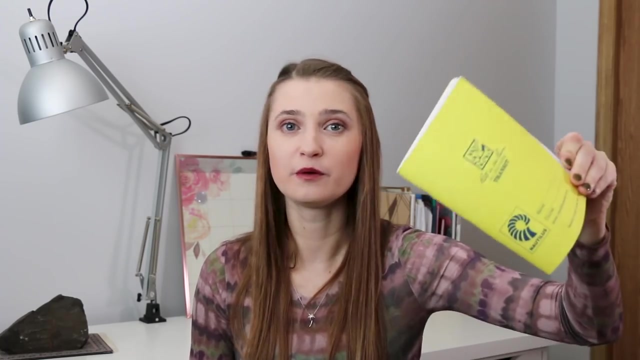 and i will be posting today a post, a geology related post, with a hammer and this notebook. if you see that post, like that post and hashtag it with hashtag shylamarocks, as in r-o-c-k-s, shylamarocks and people that are following my instagram, following this channel and hashtag. 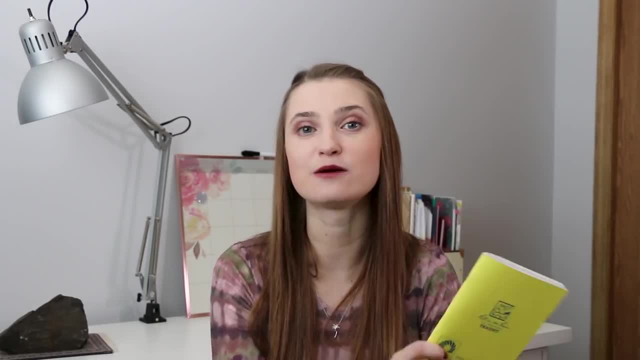 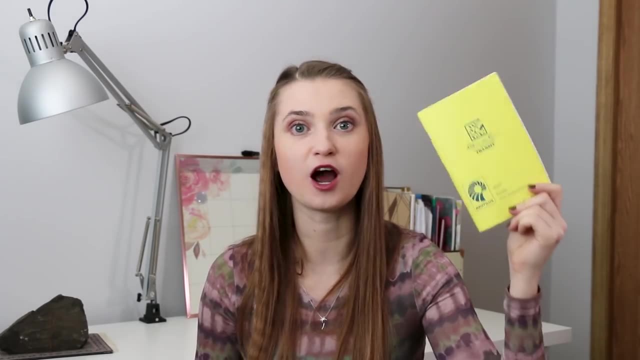 that post, i will be entered into a lottery and i will announce winner in the series number five. so when you see an episode number five, that's where i will announce the winner of for this giveaway. now, this notebook. why? what makes it so special is it's coated with. 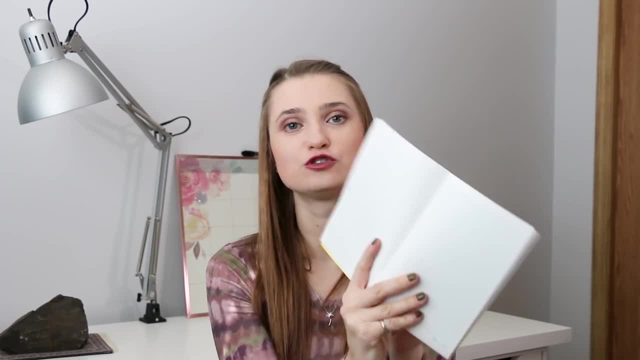 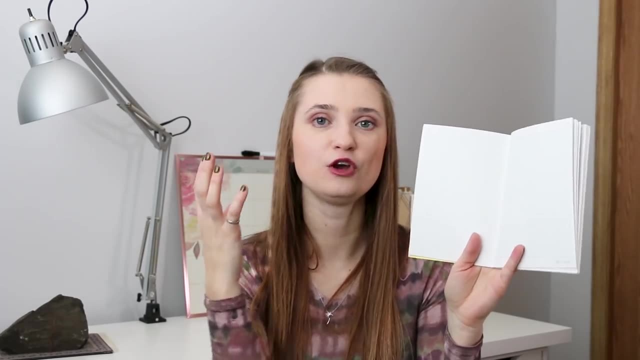 some sort of wax material. so when you're in the field and you're trying to do your notes and you're trying to draw your map, and it's raining or snowing- which often does in the mountains- um, your pages don't get ruined, they don't get wet, the ink, ink doesn't get smudged, so it's very. 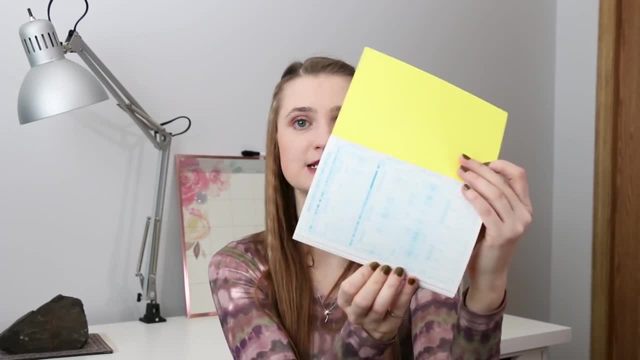 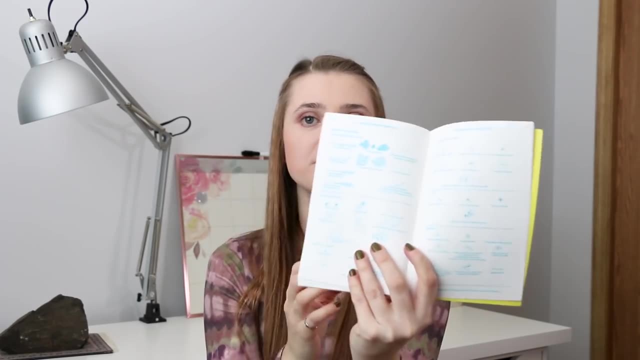 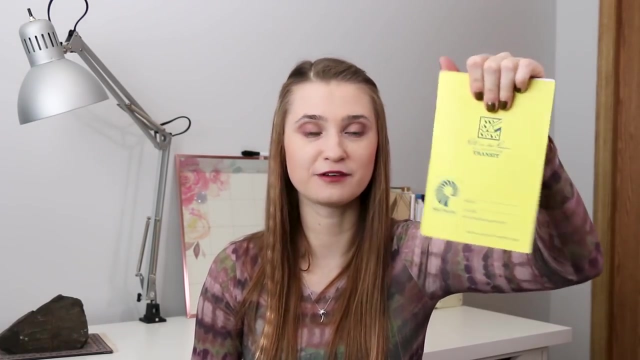 handy. it also has all the geological terms on the back. it has a time scale like a geological time scale. uh, rock classification charts, map symbols that you often use in a map if you forget them. so it just it's really handy, very useful thing to have and i've had like a million of them for. 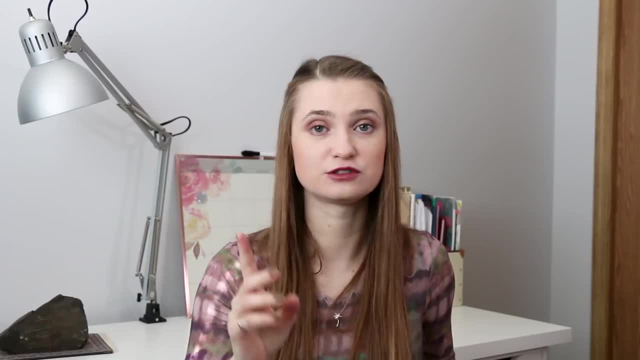 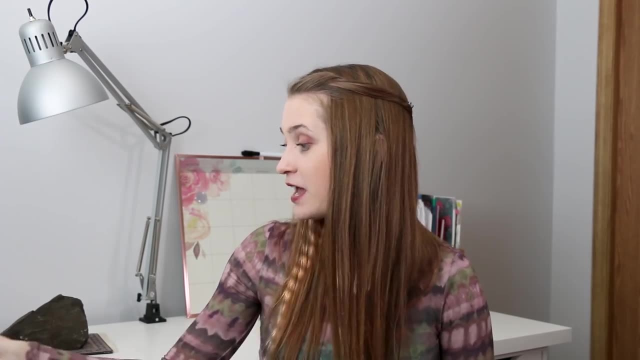 my field courses. in my um degree, i had to take four field courses and in each one of them i probably used two or three of those, because you do have to take a lot of notes to write a report now. finally, what kind of geologist would i be if i didn't collect any rocks during my field work? 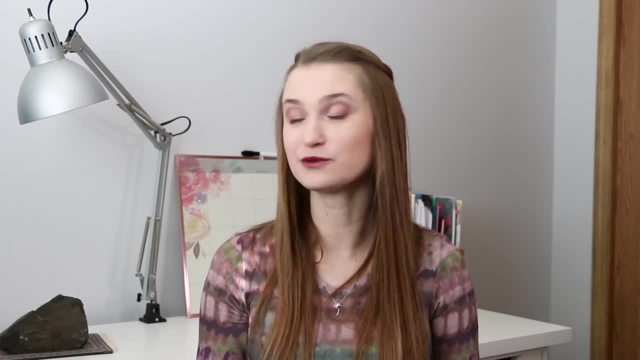 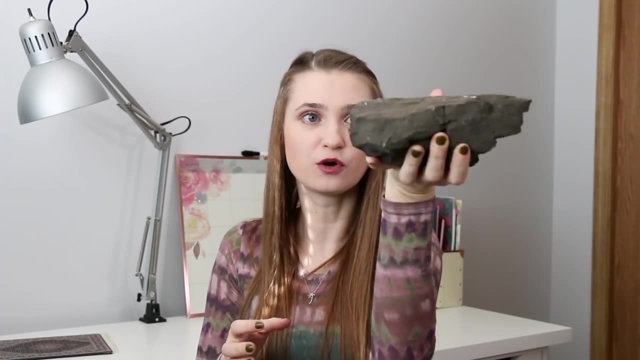 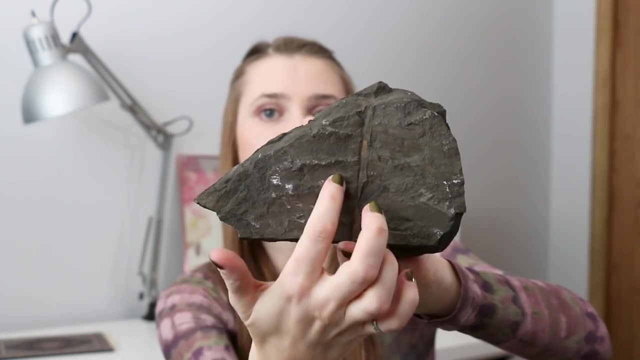 and i'm gonna show you specifically rocks i collected during my field work. so rock number one is this one. now, um, you might think there's nothing special. it's just like a hunk of siltstone, but if you look really closely it has a plant imprint. uh, here, so you see a stem and leaf imprint. 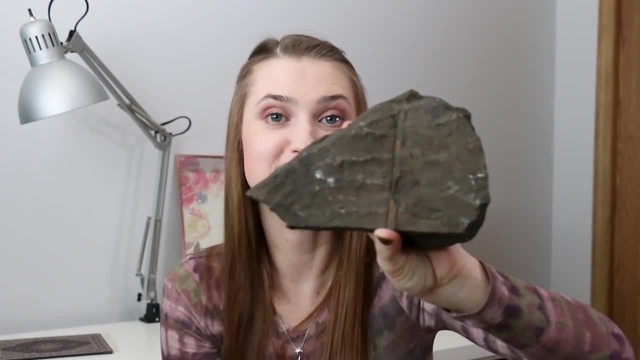 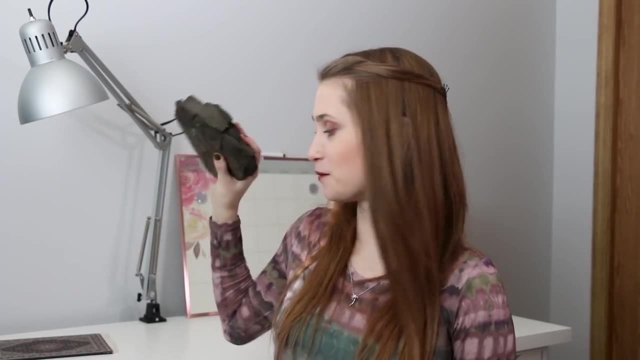 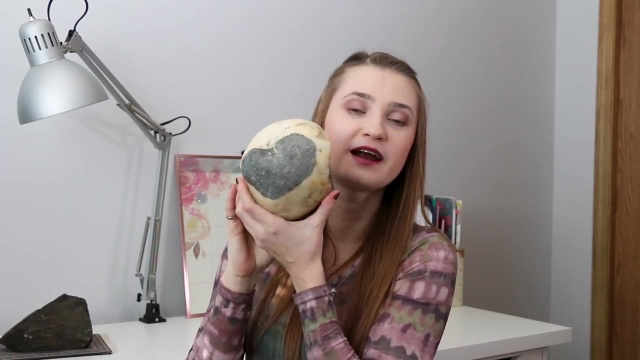 so this was my very first drug that i personally found that had a fossil in it and i thought it was really cool. i brought it back home. back then i was living with my parents. my mom was not impressed with this rock, but nevertheless i still have it. next thing is this guy. this guy is super heavy. it's. 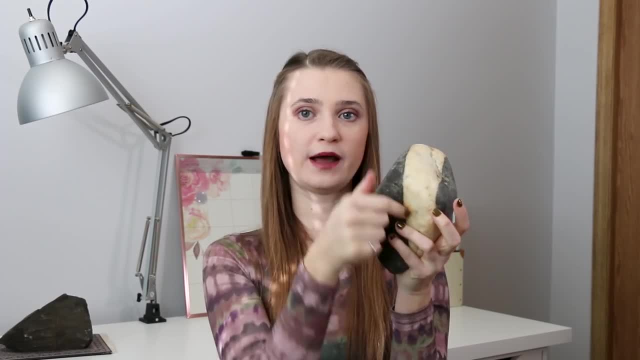 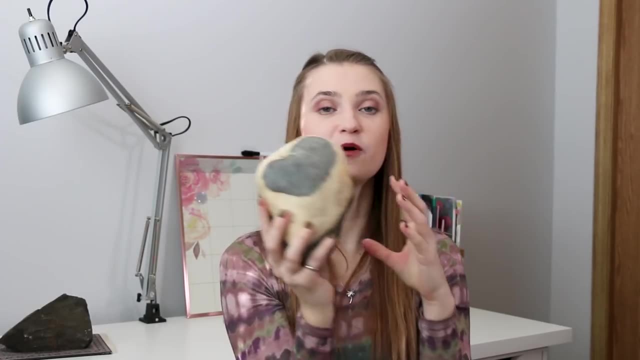 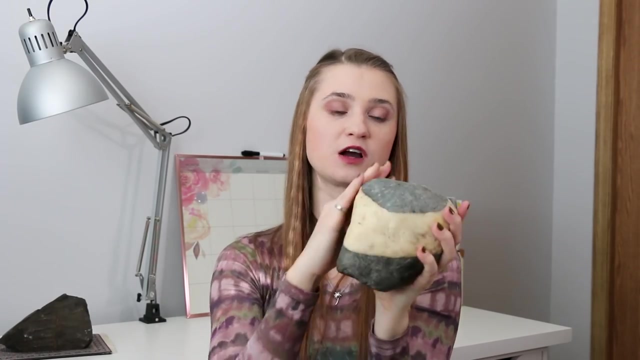 an igneous rock with a calcite vein. so this is what that white material is- is a calcite vein and it. look at this. it has a really cute heart on it. now i found this in british columbia field course. uh, we were walking down the river pass and i found this, as you can see, by this rock. it's a. 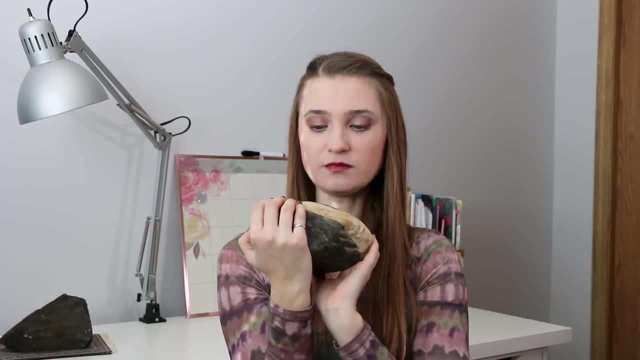 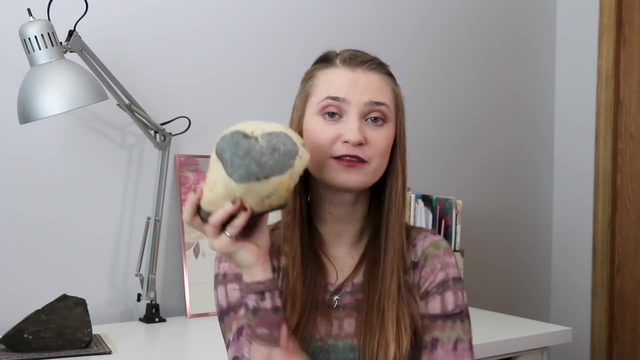 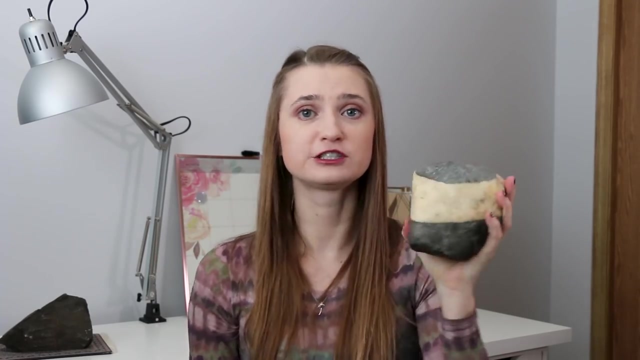 really smooth, really weathered down, so it's been under elements for quite some time, but the way it weathered it created this perfect heart shape. now this rock is really heavy and i found it on day one of my 10 day field course, so i had to lug this thing around for 10 days in my backpack. 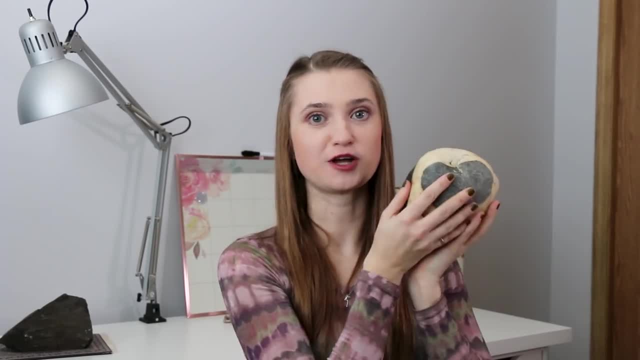 wasn't pleasant, but i did it, and now it serves as a doorstop- literally a doorstop for my balcony door during summer. next thing i have is a balcony door which is a very, very comfortable pine tree, and this is going to be my balcony product for the summer. next thing i have is a balcony door called 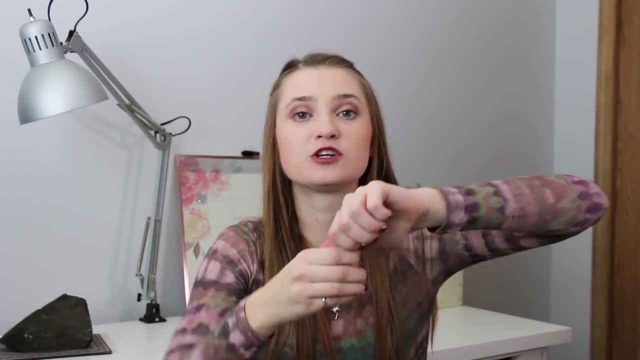 how to make a balcony door and it's really hard to open the balcony door so you can get a nice big balcony. next thing i have is a balcony door which is a really high quality and very easy to use. then we have also a balcony door. next thing i have is oil scent and, being a petroleum geologist, we did visit an open mine. 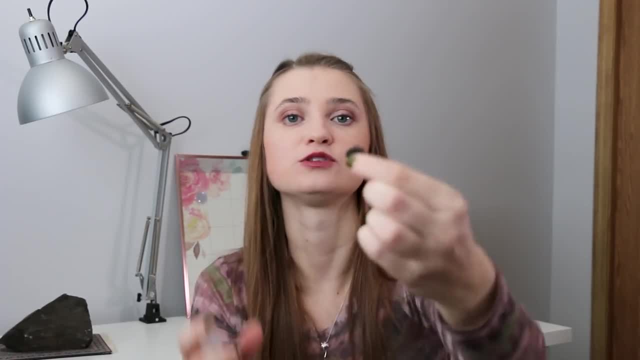 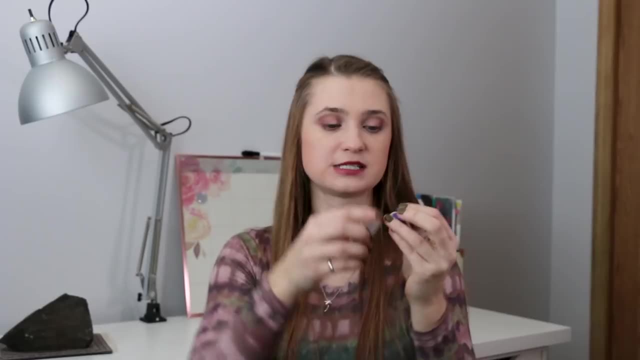 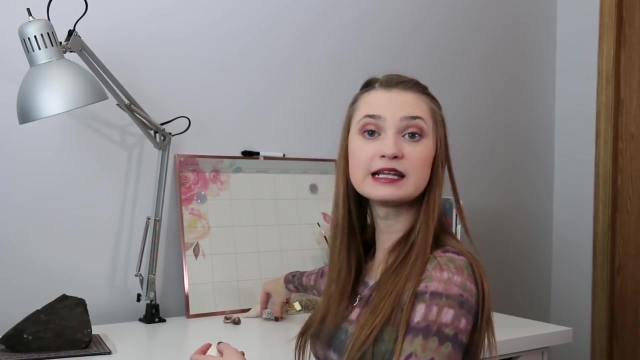 pit excavation for oil sands, and i took some samples and literally what that is is scent saturated with oil. that's all it is and that basically lives in this container. and finally, not quite a rock, but something i collected during a field course to south carolina- uh, charleston- 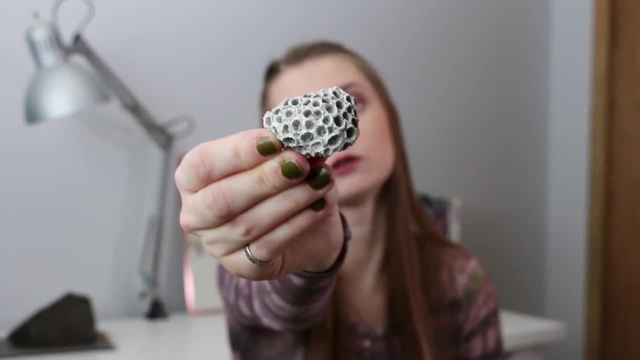 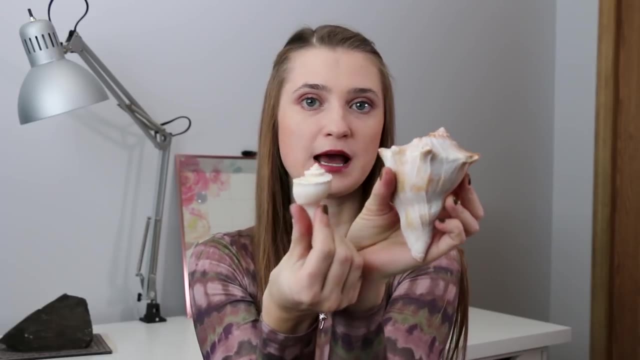 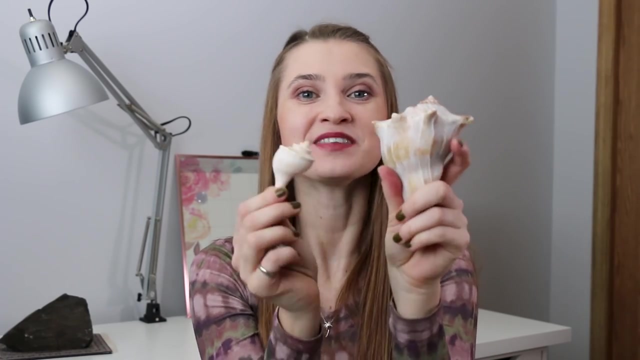 i collected a piece of coral. now it's a dead coral. i would never take a live coral out of the water. this is dead coral that was on a beach and a couple shelves that were absolutely adorable. they're not quite rocks, but they sort of fall into geopolitology field and i thought they were.